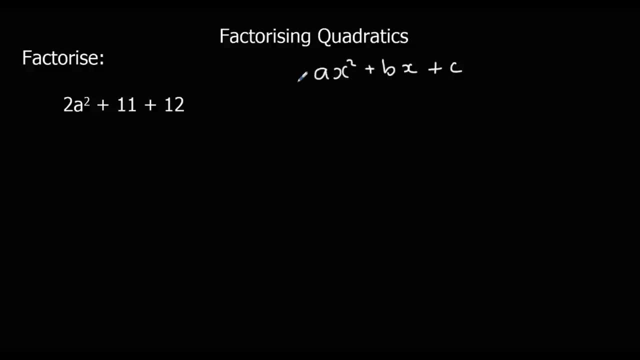 process. They are possible to do by inspection, by guessing, but I think it's easier when you're first doing it to follow a process. So that's what I'm going to show you now: a process for factorising when we've got a coefficient in front of the x squared or the. 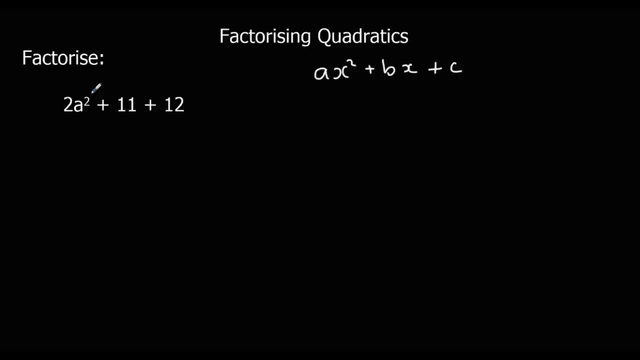 a squared. So the first step that we're going to do is we're going to take this a term and this c term. We're going to multiply them together. So 2 multiplied by 12.. So 2 twelves, that's 24.. 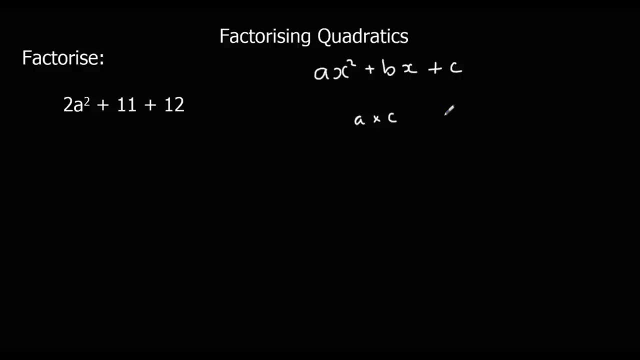 So we're going to do that a times c and that's going to give us 24.. Okay, now we're going to look at the factors of 24.. So we're looking at what multiplies to make 24.. So we can have 1 times 24,, 2 times 12,, 3 times 8,, 4 times 6, and so on. 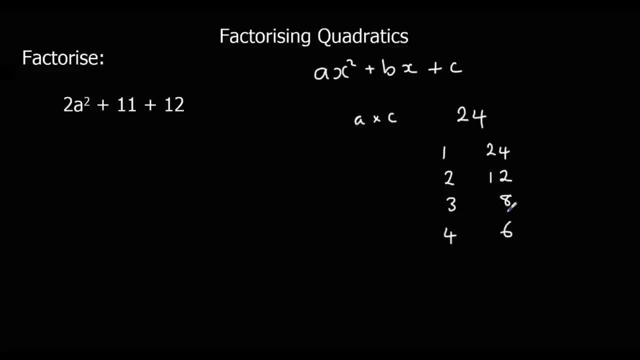 So there are no more. So they're all the factors of 24.. Then we look at: there should be an a there. Then we look at what? which of these can we get to make 11.. So which can make 11.? So 1 times 24, well, 1 and 24 can't make 11, 2 and 12 can't, 4 and 6 can't. So 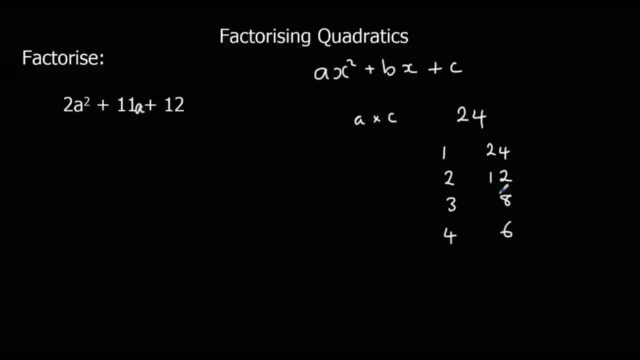 it's going to have to be 3 and 8.. So we use the 3 and 8 to rewrite this. So what we're doing here is we're unadding the two terms in the middle. When we expand, we get four terms, and then we simplify What. 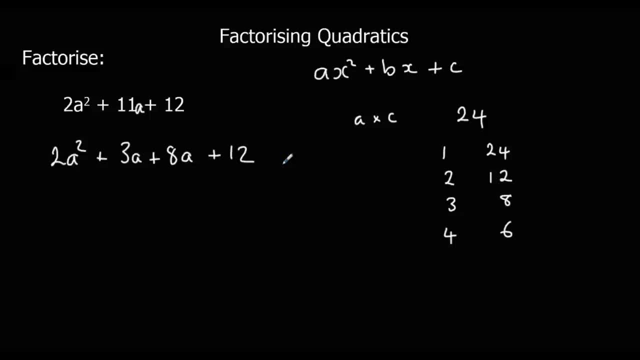 we've done. by doing that, doing the a times c, finding the factors and seeing which of those can make our b number our middle number, we've unadded those two terms that we get from expanding. Then what I'm going to do now is I'm going to cut this in half, So I'm just looking at. 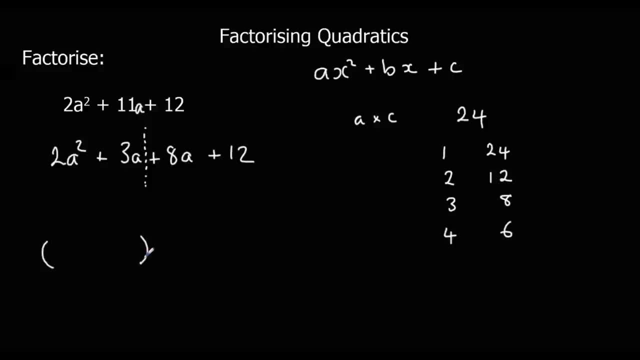 the first two terms. So what we're going to end up with is two sets of brackets like this. And do you remember when we expanded, it was the first term multiplied by both of these terms. So whatever the first term is, it makes both of these, It's a factor of both of these. 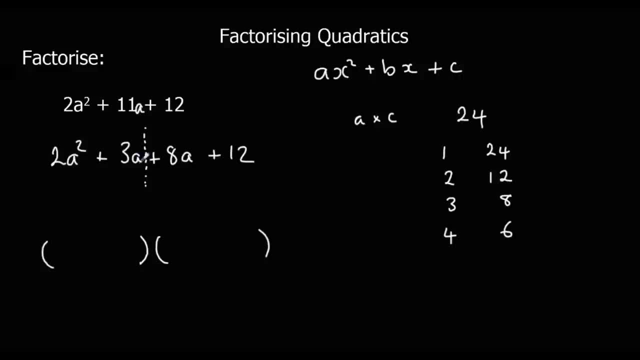 So what we're going to do is we're going to factorize just these first two terms here. So what goes into both of them? Well, we're going to factor between two and three, So it's just a. So we take a outside and 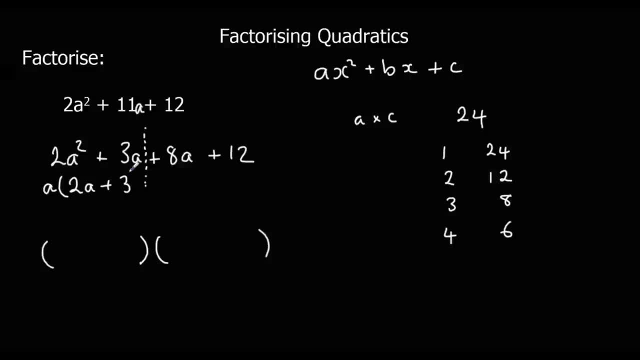 that leaves us with 2a plus 3.. So this first term, a- I'm going to put it here because that's what- multiplied by both of these terms, We're going to factorize the second part as well, And we've got 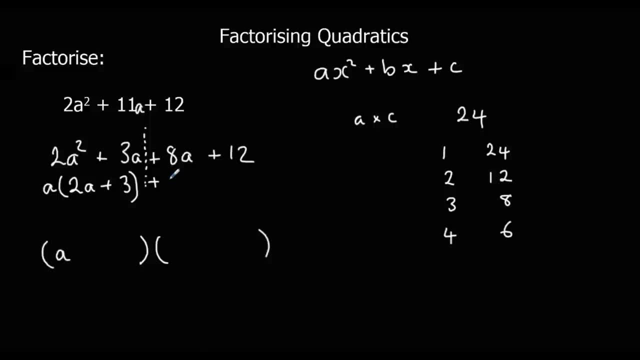 8 and 20.. 8 and 20. 12.. So the common factor there is 4.. And 2a 4 times 2a makes 8a, 4 times 3 makes 12.. So we've got the same bracket here and here, which is good. That's what we wanted. 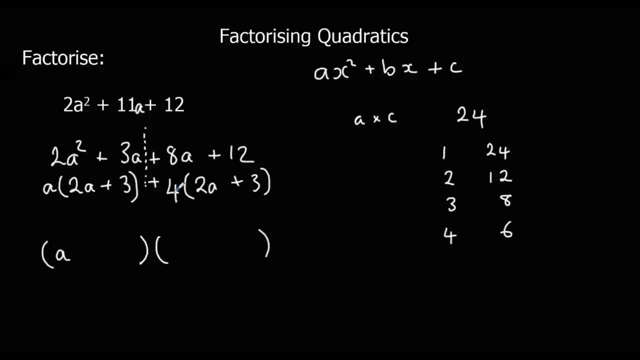 We've got a multiplied by both of these and then 4 multiplied by both of these. Now, this is just another way of writing: a plus 4 and 2a plus 3.. we've got a times both of them, which is the first half, and then four times both of them. that's the. 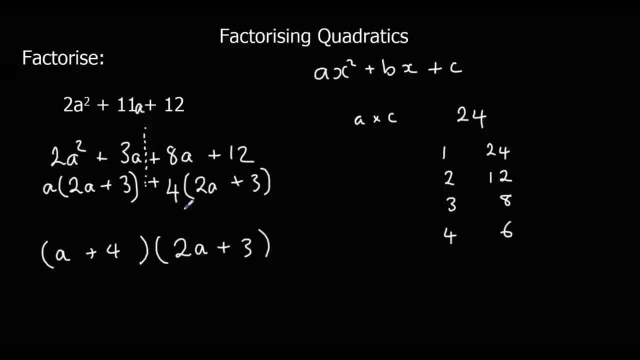 second half. so this is just a way of rewriting the same thing. so this means this and this is factorized and this is our final answer. so here's another question. we're just going to follow the same steps. so it's a times c, first the first, one times, the last one, two times. well, it's minus five. 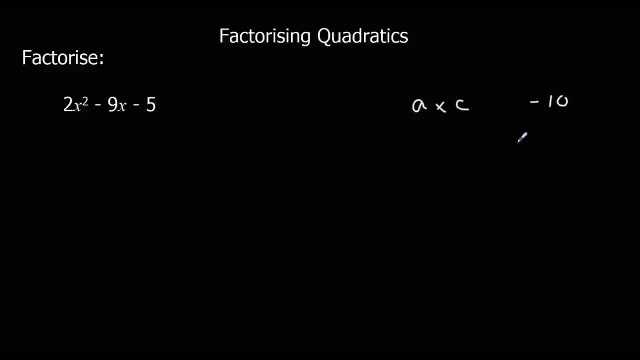 so it's minus 10. but we can ignore the minus. largely it's just um. it's worth noting that it is a negative, so it's factors of 10. now, so a times c minus 10, the factors of 10. so 1 times 10 or 2. 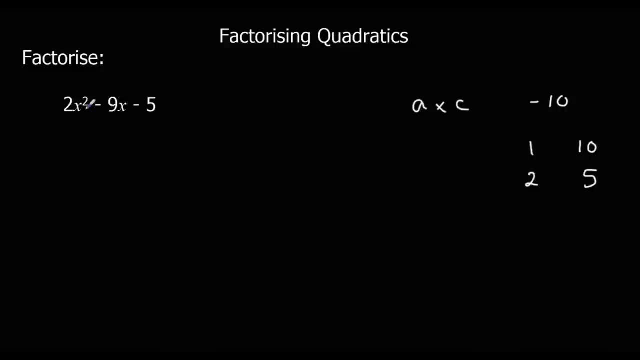 times 5. we need to make a 9, so it's going to be 1 and 10 and it's a minus 9, so we're going to have minus 10, 10 minus 10x plus 1x. so we've just rewritten minus 9 as minus 10 plus 1, so we've undone the adding up that we did from. 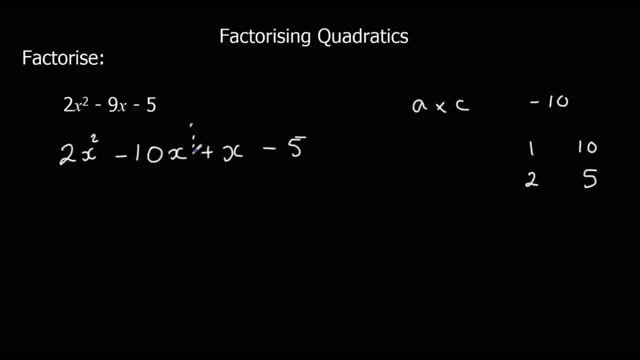 it that we get from expanding. cut it down the middle, we factorize the first half, so that's going to be common factor between 2 and 10 is 2 and they've both got an x. 2x times x makes 2x. squared, 2x times minus 5 makes minus 10x. so we start to form our brackets. 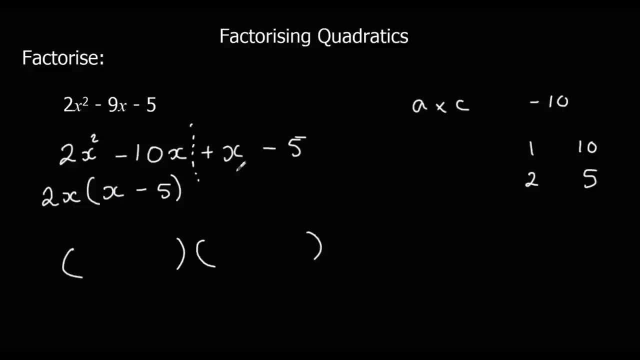 we know the second bracket here is going to have to be the same. so this is x minus 5. and what's left here? well, there's no common factor, so it's just 1. so we have 2x plus 1 and we have x minus 5. 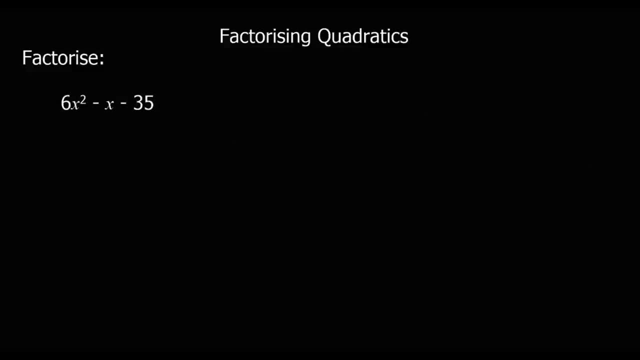 that's the final answer. okay, this is. i've deliberately made the numbers difficult in this question, so we're going to do a times c, so it's 6 times 35. so a times c, 6 times 35, that's 210, it's a minus 210. i'll put the 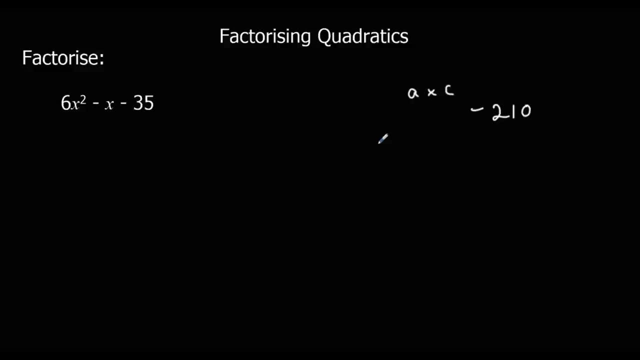 minus there. then we have to look at the factors of 210. so there's going to be a few um. it's 1 times 210, 2 times 105, 3 times 70. it's not in the four times table. it is in the five times table. that would be. 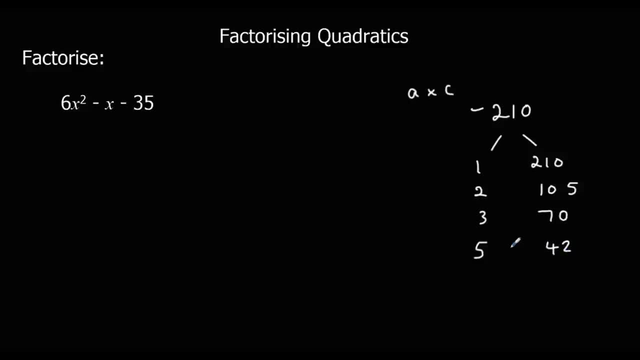 42 times. it is in the six times table um 35 times, 7, 30 times. it's not in the eights, it's not in the nines, it's in the 10 times table 21 times. it'll be in the 15 times table 14 times. so it was in the 14 times table. 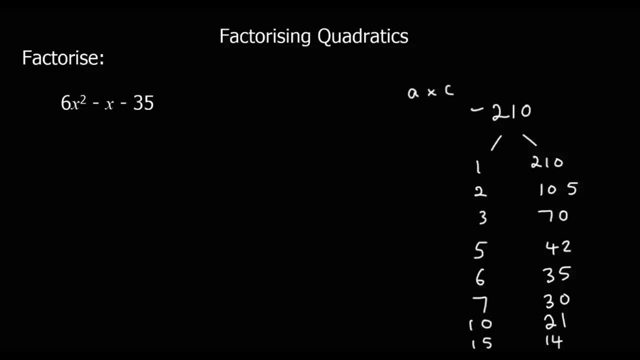 um. so which of these can make a minus 1? it's 15 times 14.. so we've got 6x squared minus 15x plus 14x. that makes minus 1 minus 35. so we've rewritten this and then we cut it down the middle common factor between 6 and 15: 3, and they've both got an x. 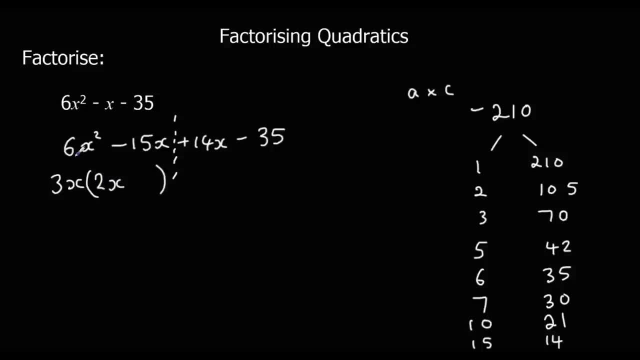 so we've got 3x plus 7 plus 7 and 3x plus 2 and 3x plus 3x, and 3x times 2x makes six x squared, and 3x times minus five makes minus 15.. second bracket: we know it's going to be 2x minus 5 and 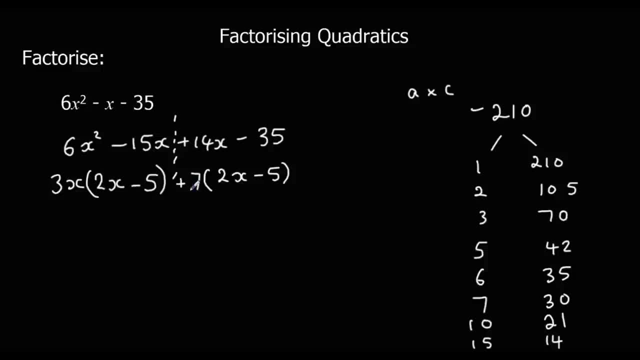 what multiplies by these terms to make that it's 7.. so 7 times 2x makes 14x. 7 times minus 5 makes minus 35.. so the first bracket is 3x plus 7.. and the second one is 2x minus 5. again, you could have got this with the two. 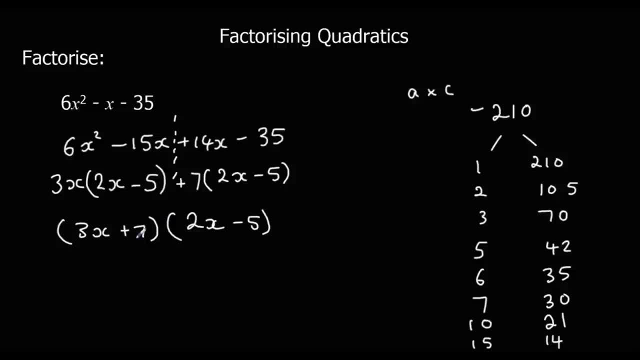 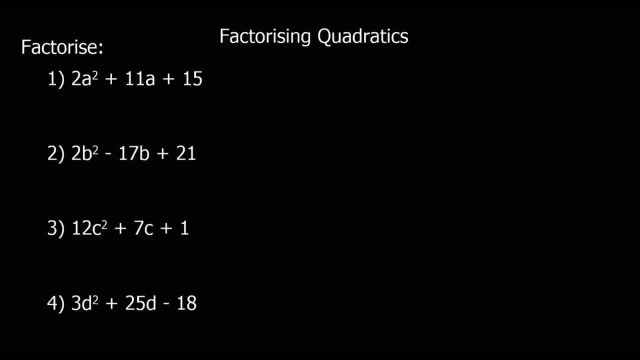 brackets the other way around and it would still be right. so that is the answer to that one. okay, here's four questions. pause the video and have a go at them, and just follow the same process a times C: rewrite it, cut it down the middle, factorize each half. so give them a go and I'll put the answer up. 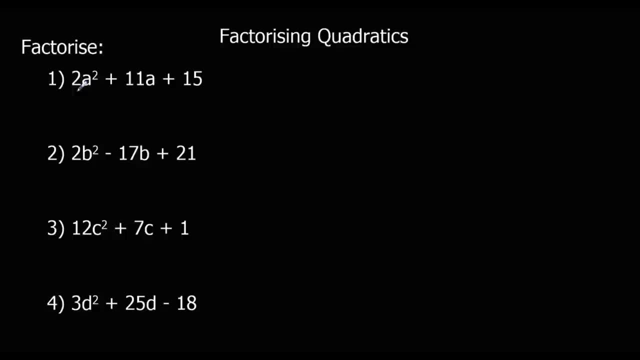 afterwards. okay, the first one so we should have a times C is 30. so a times C and we get 30 and the factors of 30 that make 11. we should have got 5 and 6, so 2 a squared plus 5 a plus 6 a plus 15. if you've written the 5 a and the 6 a, the 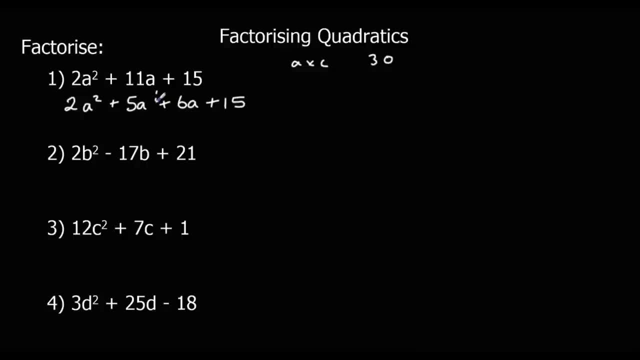 other way around. that's okay, you still get the same answer at the end. you so factorize the first half. so take out a 2a plus 5, 2a plus 5 and this is a plus 3. so the two brackets should be a plus 3 and 2a plus 5, second one. so a times C is. 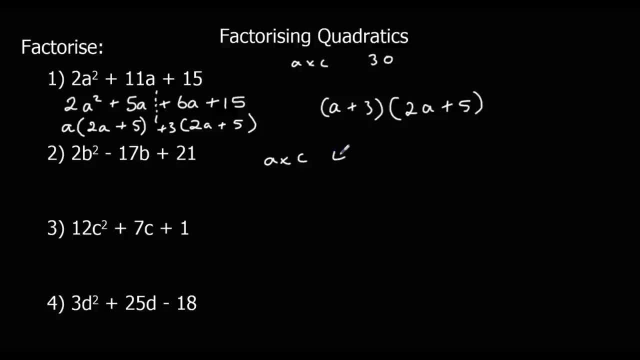 42 A times C 42, then the factors of 42 that make minus 17, that would be 14 and 3. so 2b squared minus 14b, minus 3b plus 21, cutting it down the middle, taking 2b out the first bracket, and then I've got b minus 7, b minus 7 again here. 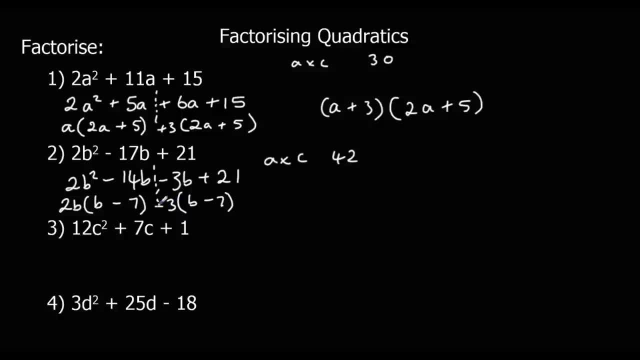 what's going to make this? if I multiply by minus 3 minus 3 times b is minus 3b minus 3 times minus 7 plus 21. so our two brackets are 2b minus 3 and b minus 7. thirdly, we've got a times c is 12. 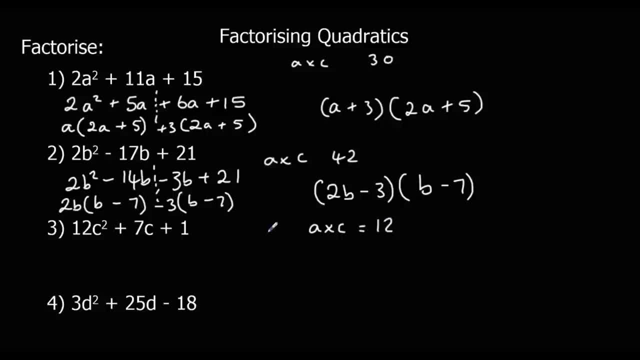 12. which factors are we looking for? it's 3 plus 4, so 12 c squared plus 3c plus 4c plus 1. cutting it again, take 3c out, the first bracket leaves 4c plus 1, 4c plus 1 and that's just one. so 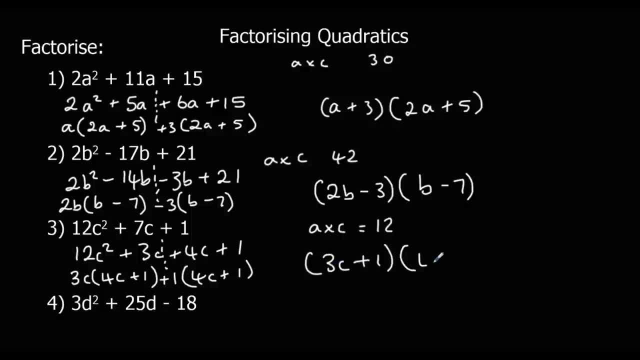 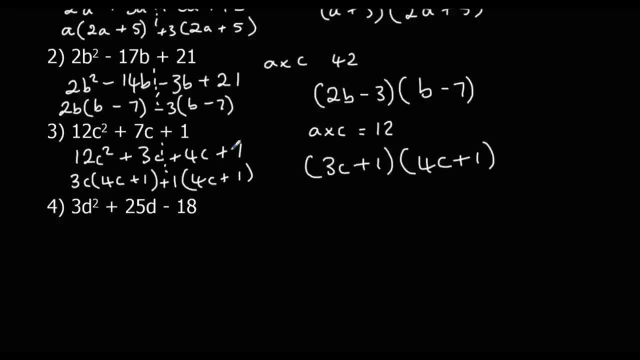 the two brackets, 3c plus 1 and 4c plus 1. okay, the last one. I've got a times c, and that is 18 times 354. factors are 54. um, that make 25 is going to be. well, let's write them out so. 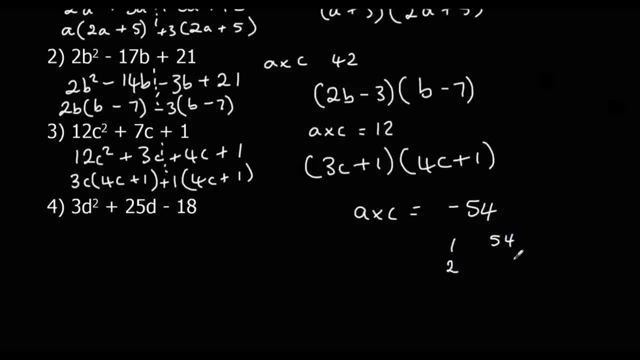 we could have 1 times 54, 2 times 27, 3 times 18, and is it in the fours? no, it's not in the fours, not in the fives. 6 times 9, 9, and they are all the factors. so we're going to use 2 and 27. we can make 25 out of 2 and 27, so 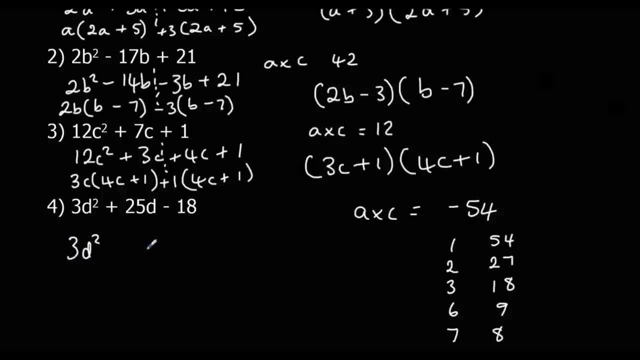 we're going to rewrite it as 3d squared plus 27, D minus 2d minus 18, cutting it down the middle, so 3d on the outside, which leaves D plus 9 and a B plus 9 in the second one. and that's not whether. 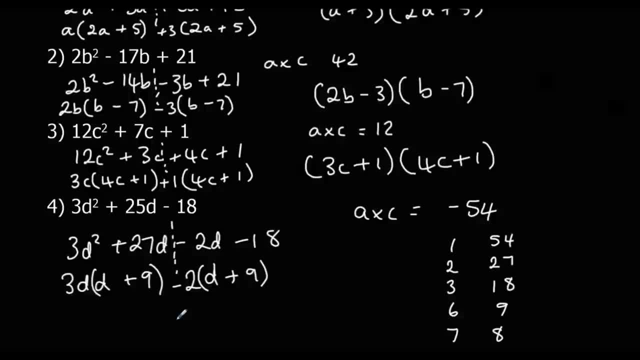 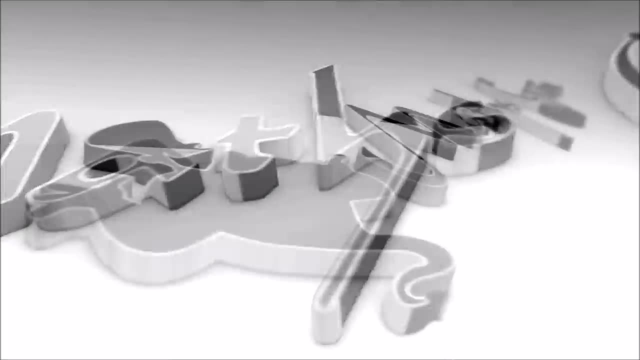 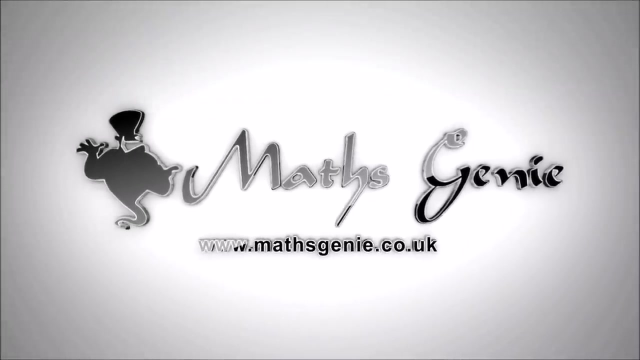 that. multiply that by minus 2, so our two brackets are going to be 3d minus 2 and D plus 9. so just for the demonstration, we're going to cut it down Ad. 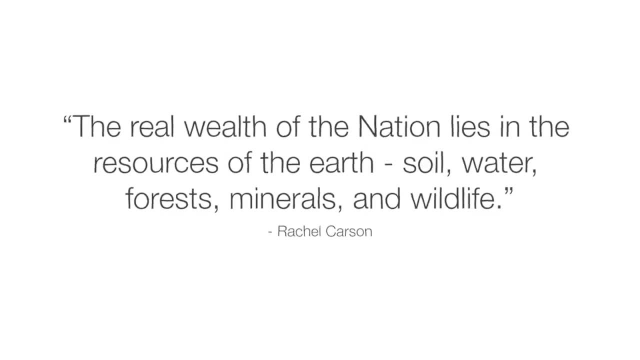 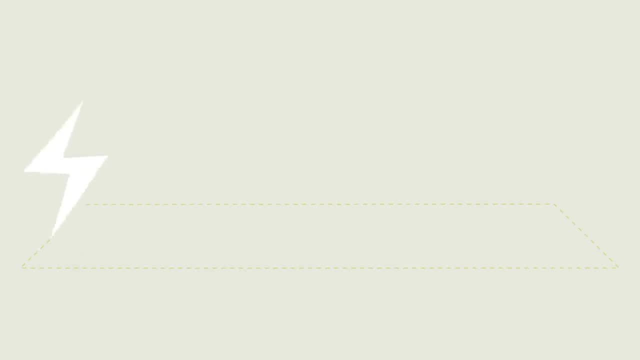 No matter how we make electricity, it takes up space. Electricity from coal requires mines and plants to burn it and convert the heat into electricity. Nuclear power takes uranium mines, facilities to refine the uranium, a reactor and a place to store the spent fuel safely. 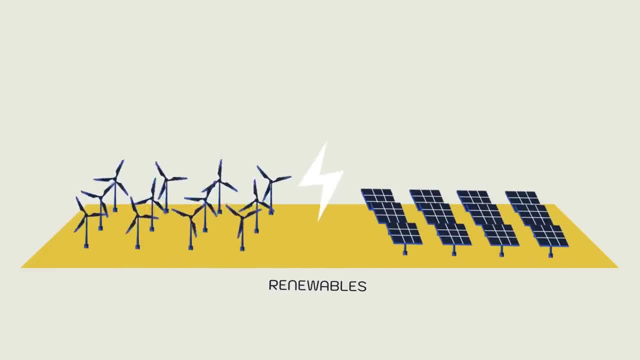 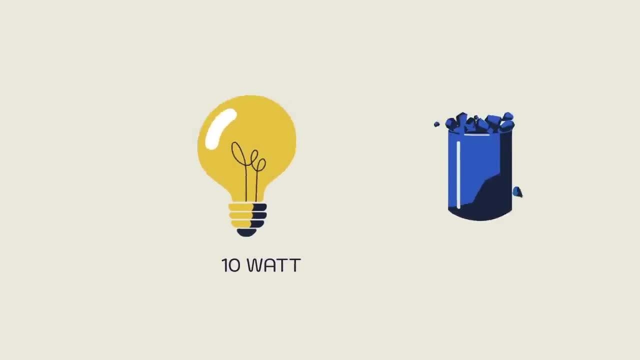 Renewable energy needs wind turbines or solar panels. How much space depends on the power source. Say you wanted to power a 10-watt light bulb with fossil fuels like coal. Fossil fuels can produce up to 2,000 watts per square meter. 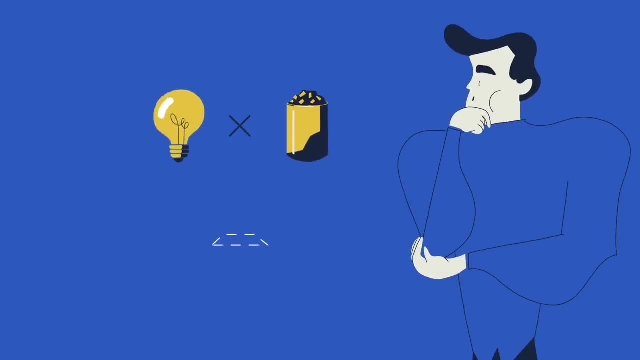 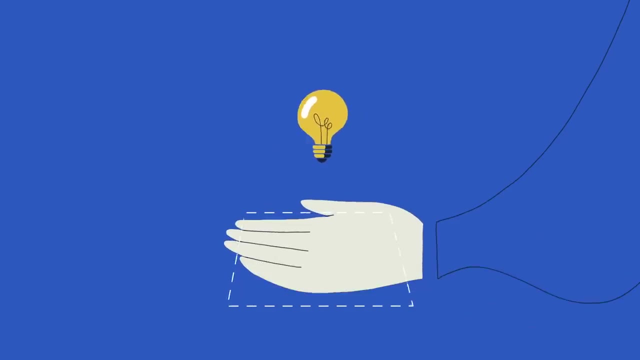 so it would only take a credit card-sized chunk of land to power the light bulb. With nuclear power, you might only need an area about the size of the palms of your hands. With solar power you need at least 0.2.. 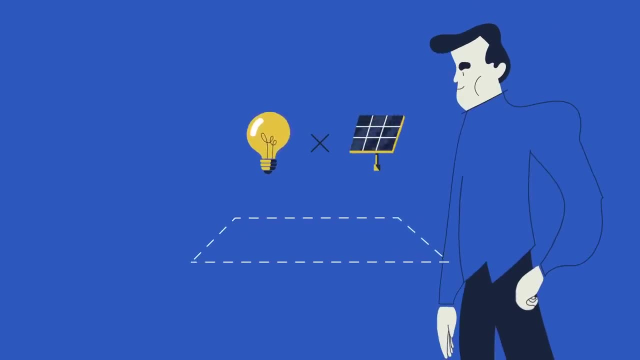 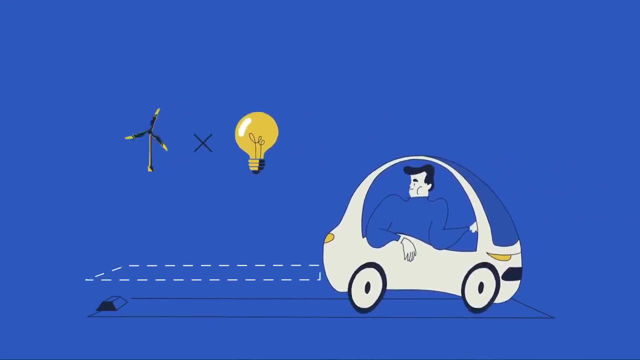 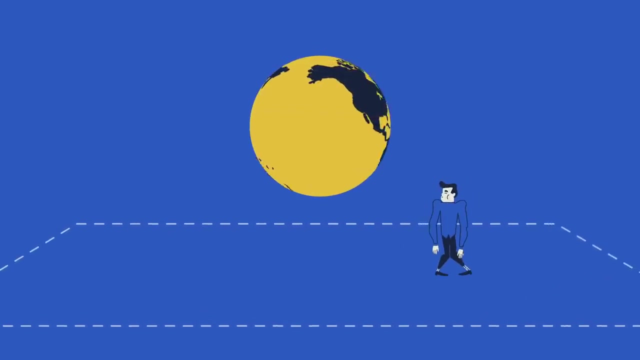 That's 1.3 square meters of land, twice the size of a cafeteria tray. Wind power would take roughly 7 square meters, about half the size of a parking space, to power the bulb, When you consider the space needed to power cities, countries and the whole world. 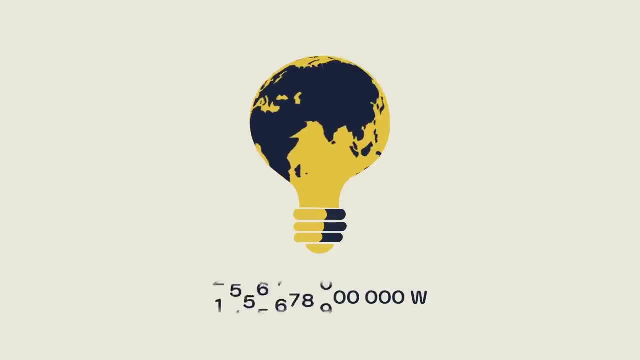 it adds up fast. Today the world uses 3 trillion watts of electricity. To power the entire world with only fossil fuels, you'd need at least about 400 square kilometers of space, roughly the area of Grand Bahama Island. With nuclear energy, you'd need almost four times as much space. at a minimum.